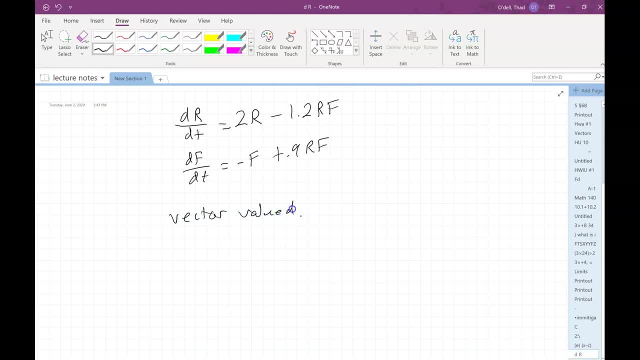 Vector-valued functions. So a vector-valued function is a function that's based on a vector rather than an equation. Of course, the vector could have equations within as the terms of the vector. So what we're going to do is we're going to take 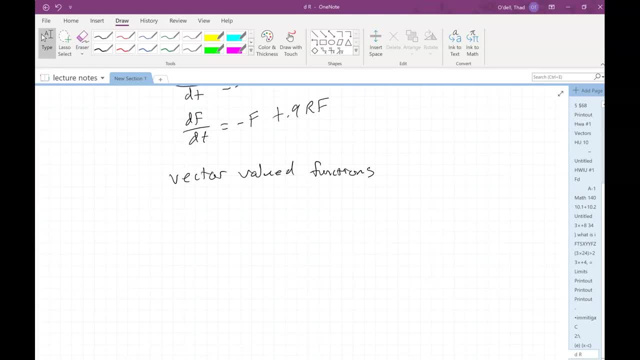 so if we're looking for solutions, this equation we're going to create a solution that's made up of it's a vector-valued solution, that is so. let's say p of t is my solution. p of t is equal to the vector r of t, f of t. 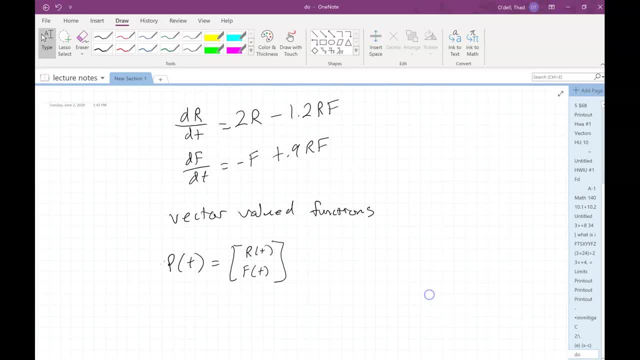 So again, that means r of t would be the solution. so we're going to take the solution to this equation. well, they actually both are solutions. So in other words, we're saying, if we plug in r of t there, there and take the derivative of there, 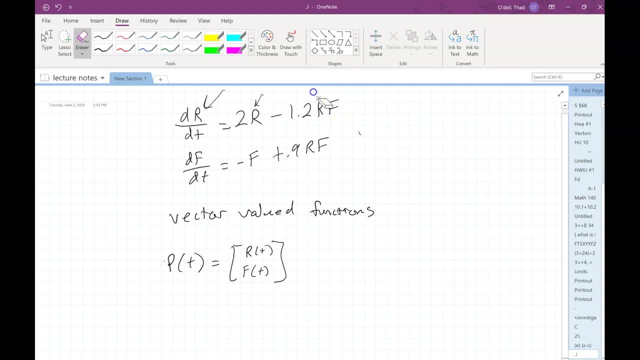 and plug f of t in here. let's use colors. this arrows are lame. Okay, so we're saying so. here's r of t. so that means it would go there, there, there and there. Here's f of t that would go there, there, there and there. 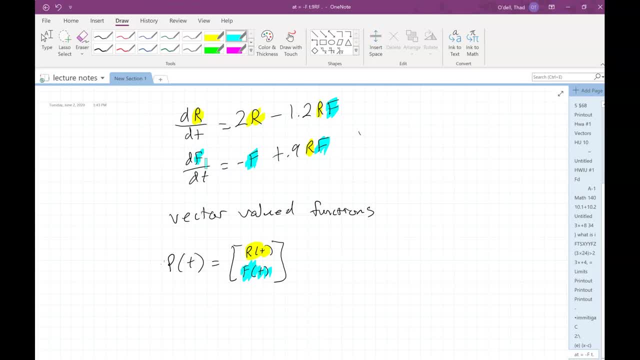 So what we're saying is that r of t and f of t are the solutions, or they together is the solution to this differential system, the differential equations. So that means that we could call this the p, the solutions, vector, okay, or vector-valued function, I mean. 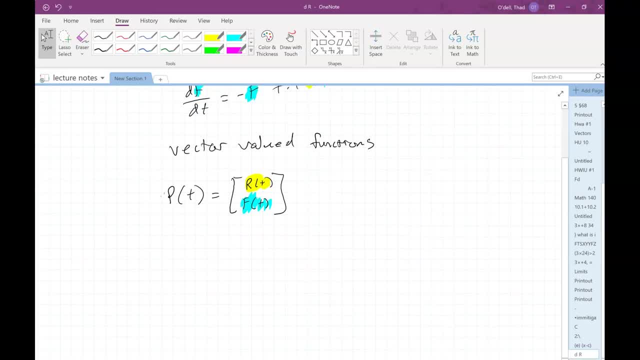 Okay, so if we know that, that, if we know that this is true, then we could also do this. We could take the derivative of p of t. of course, you can take the derivative of vector-valued function, which would give you dr- dt and df- dt. 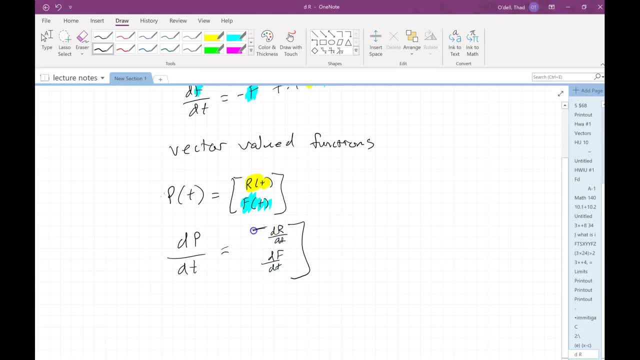 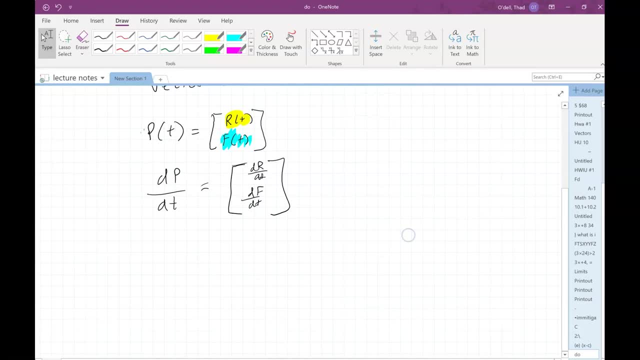 So this right here represents the derivative of the vector-valued function, which is the solution to this differential equation. And of course we know what dr, dt and df dt is. so we can rewrite dv dt as- and we'll have to make this a little bigger- 2r minus 1.2 rf and negative f. 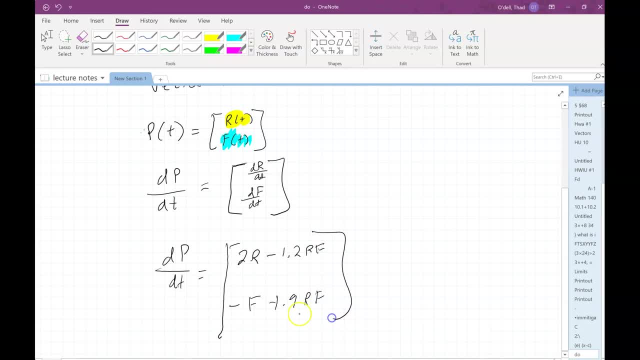 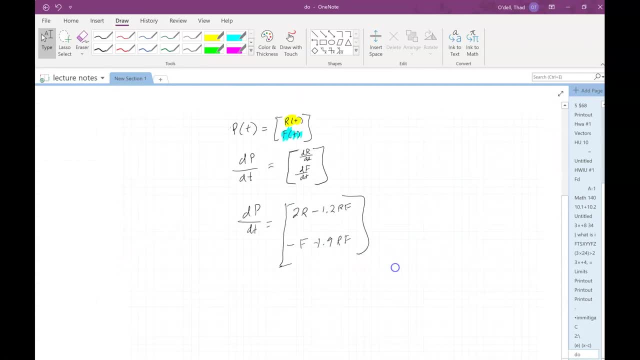 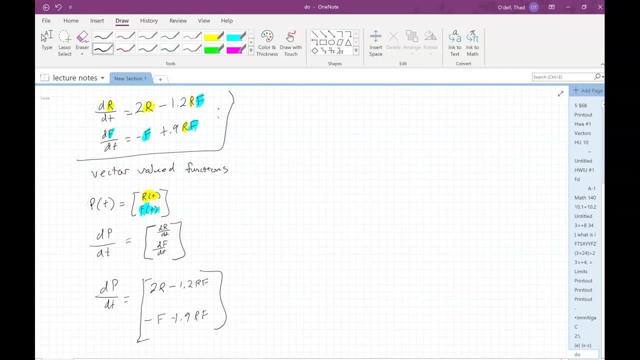 plus 0.9 rf. So that would be- and of course this just came from the original function. in case you didn't remember the original differential equations, You can see that we just replaced dr dt with what this says it is and df dt with what that says it is. Okay now. so what we're going to? 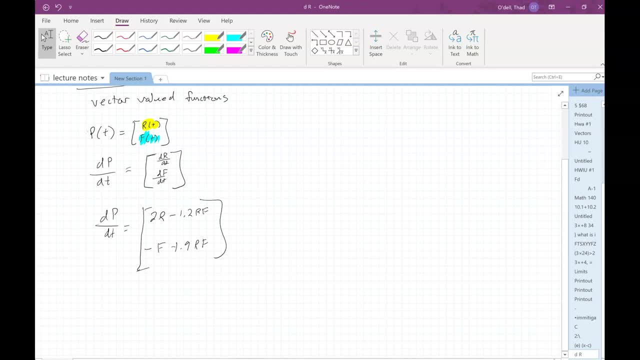 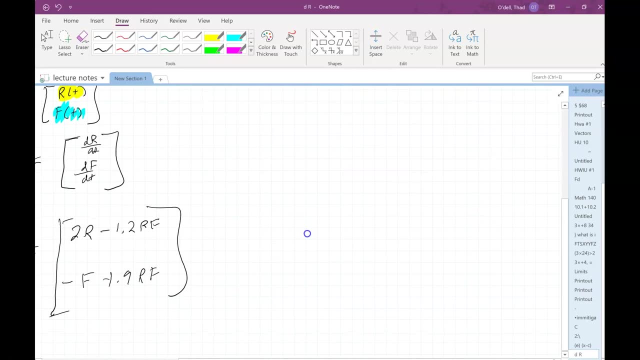 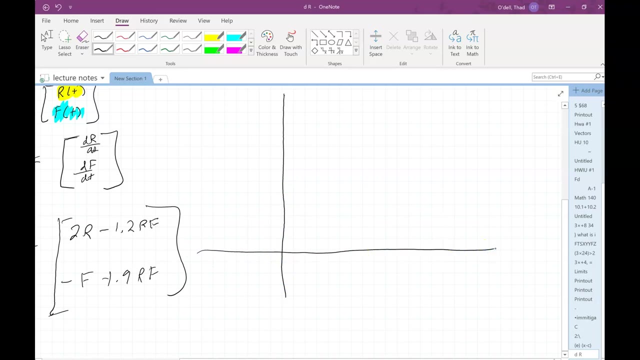 what the vector field does is it assigns a vector to each point in the field, very similar to the slope fields we had before. So if we take a, take a nice big plane, and in this plane we're going to call this the r or the rabbit axis. 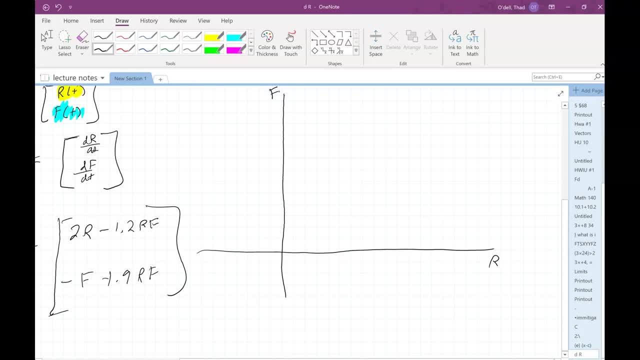 and this is the f or the fox axis. And if we pick some random point like 2 comma 1, and put a little dot there? So we want to know that if, if the rabbit population was 2 and the fox population was 1, what would these differential equations, the solution to the differential equation? 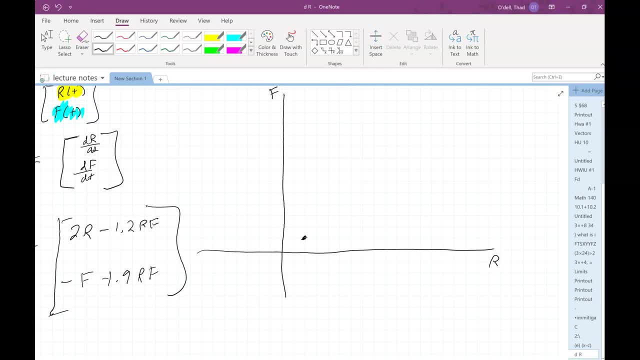 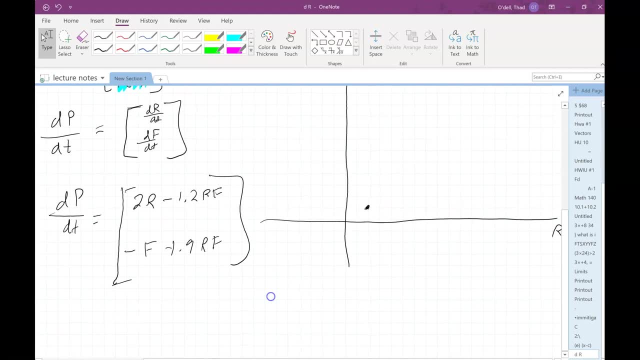 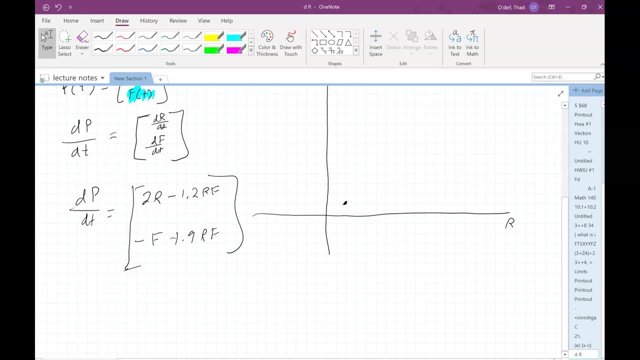 look like trying to get at right. so, um, so, in each point we can, we can assign a vector to that point. that's what this thing here is doing, and that vector would represent the derivative of the solution, which would, which would basically be a directional vector for the solution. so, um, 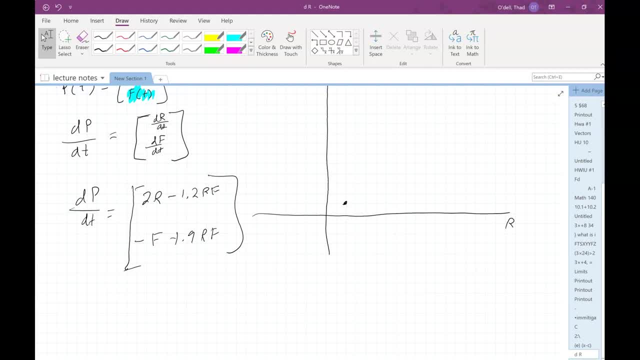 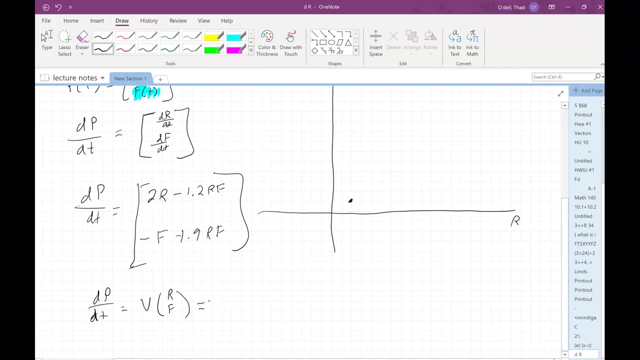 let's do this. so, in other words, i would want to know what um? so let's just, let's just make this to cut back on the uh rotation. we'll call this v of t of g. no, we'll call this v of some point, um. okay, because now the uh derivative is being represented as a, as a vector. so 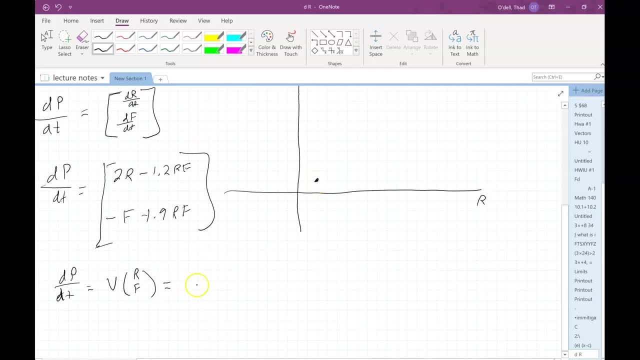 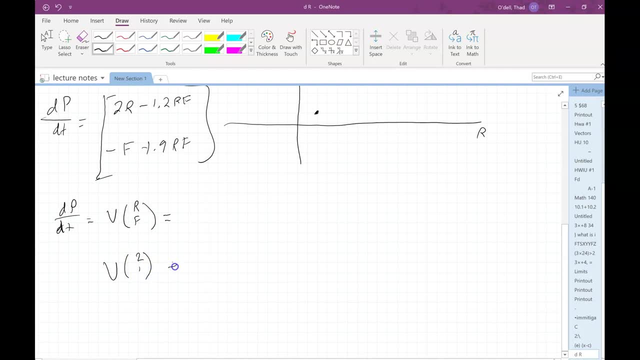 for example, if we want to know what the what it is, at this point we would say um, we would say v of two, one, because the rabbit population is two, the fox population is one. so we're plugging into this vector divide function and we could calculate a vector. 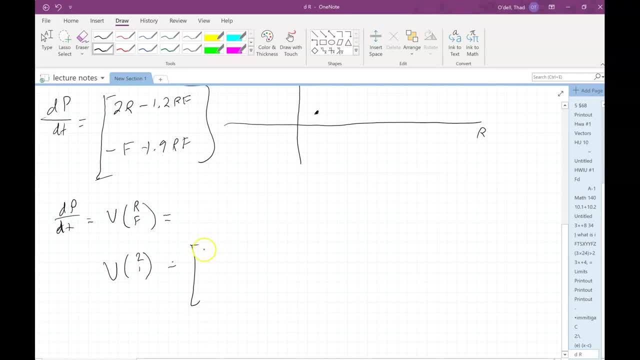 so that i should make a little bit more room there. that would be uh, 2 times 2 minus 1.2 times 2 times 1, and that would be negative 1 plus 0.9 times 2 times 1, which of course would give me: 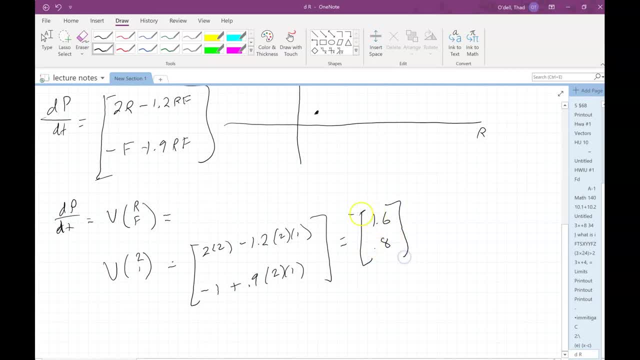 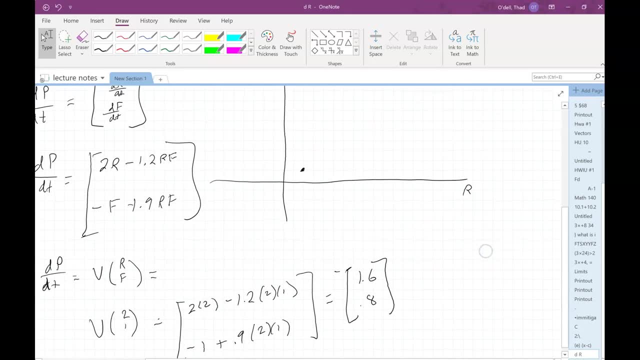 1.6 and 0.8. so now we have a vector that represents the direction of the solution at that point. so we could go up here and we could draw a vector. uh, looks like it's going in the rabbit direction 1.6, so that'd be 1.6-ish. 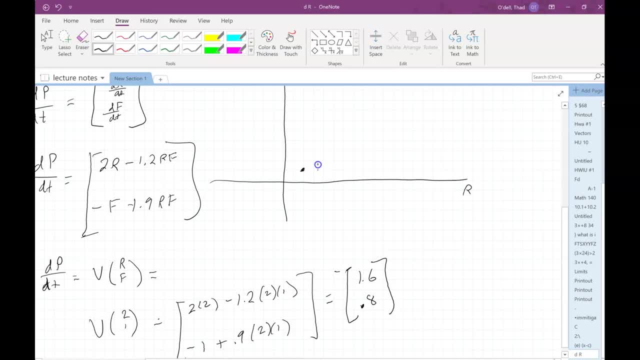 and we're going in the fox direction, point eight-ish. so it'd be right about there. so my vector is going to be like that. so that would. that is the direction, um, the uh. that gives us a kind of a directional idea of what's happening. so it looks like the. at that point the rabbit population is growing. 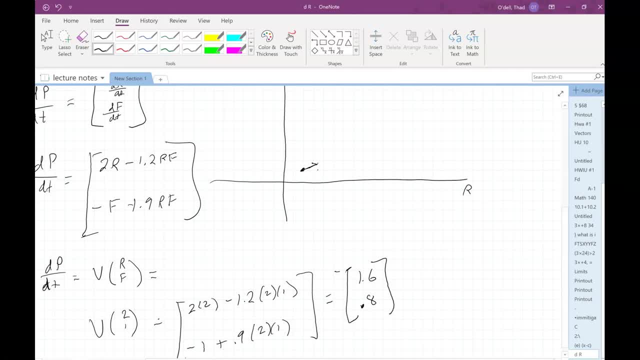 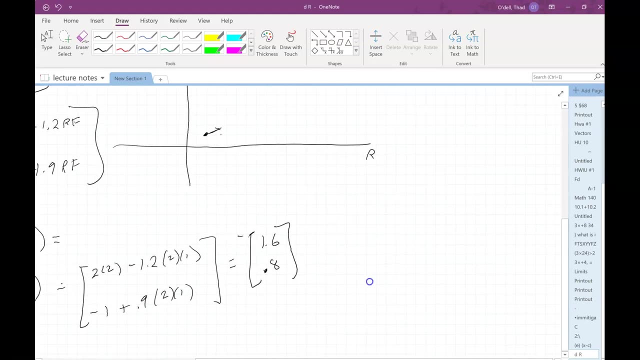 and the fox population is growing, But the rabbit population is growing a little faster. That's what that vector is telling us, if that makes sense, Because this vector in this case is really comparing the growth rates of the two populations. So then we could calculate another one like, for example: what's the vector evaluated at 1,, 1,, for example? 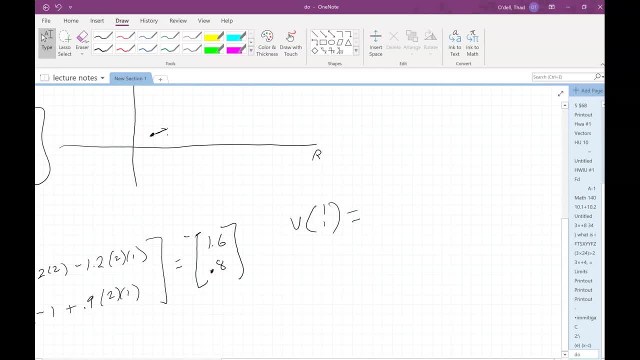 So that would be if we again plug it into the same formula, we would get the vector 0.8 and negative 0.1.. That's interesting. We're not that far away. We're over here at 1, 1.. 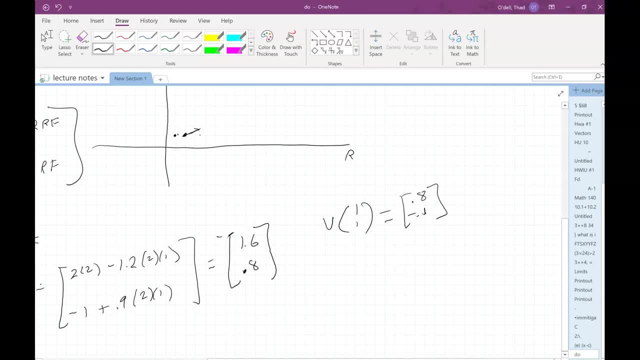 And the vector is very different, isn't it? So at that point we're going 0.8 in the rabbit direction, but negative 0.1 in the. so you can see, right about there, It blows up a little bit. 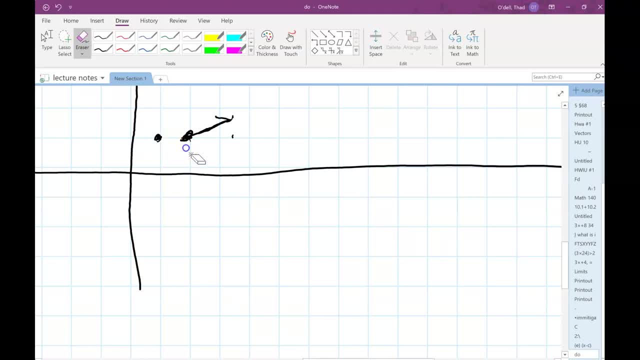 That was way too small. Let's do this again. Here we're going to go 8 and negative 1, so right about there. So you can see that if we keep doing this, we're going to get pretty crowded with vectors all over the place.